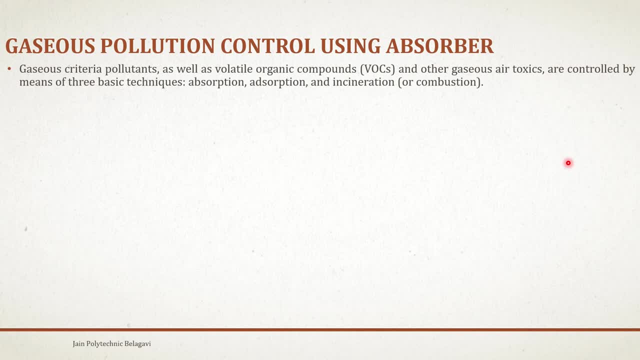 If you are going to add full glass of water with a teaspoon, one teaspoon of salt or a one teaspoon of sugar, it starts mingling with each other, in the sense the water it's been absorbed, all this sugar and the salt. Similarly, when it comes to adsorption: adsorption it is the substances which is going to just settle on the surface of the material. 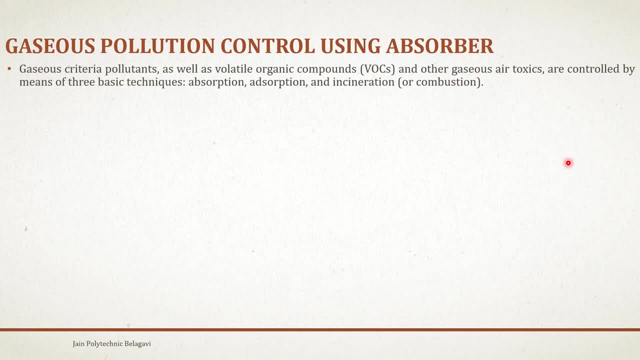 Just like if you are going to apply the powder on your face, we say it as the adsorption. Similarly, the incineration. Incineration in the sense: whatever the material is there, we are going to burn it and if that burning, we are going to check it out using saying that whatever the burnt material, it will be there, it will be evaporated and we will be cooling it down. 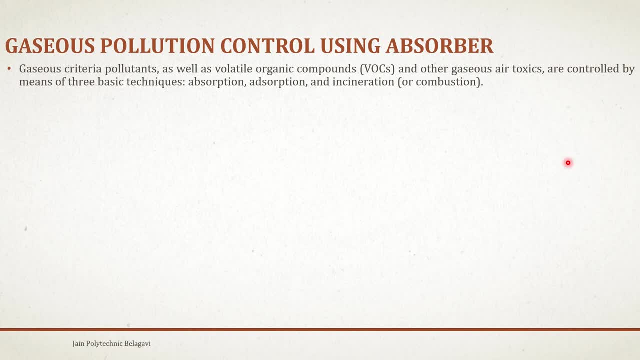 We will be settling it. we use it for other purposes. we said that it as the combustion or the incineration, So we will discuss in the context of air pollution control. absorption involves the transfer of a gaseous pollutant from the air into a contacting liquid such as water. 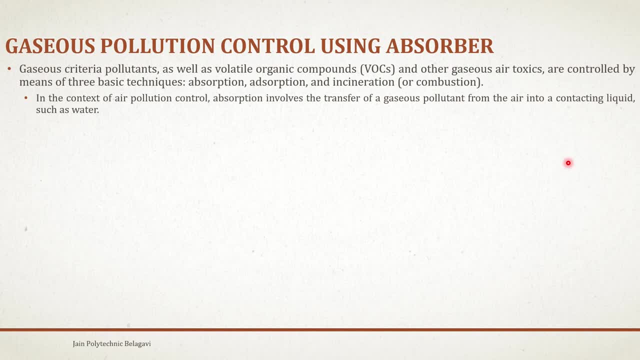 As I have given you the example Here, the water. it will be absorbing The pollutant from the gas. Next, we have different instruments for absorption technique: Wet scrubber and the packed scrubber. These described above for controlling suspended particles may be used for gas absorption. 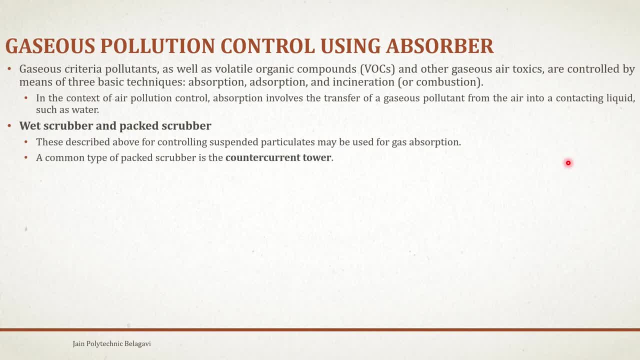 A common type of packed scrubber is the counter current tower. The liquid absorbent flows downward and is uniformly spread throughout the column packing. These devices usually have gas removal efficiency of 90 to 95%. So this is about the wet scrubber and the packed scrubber. 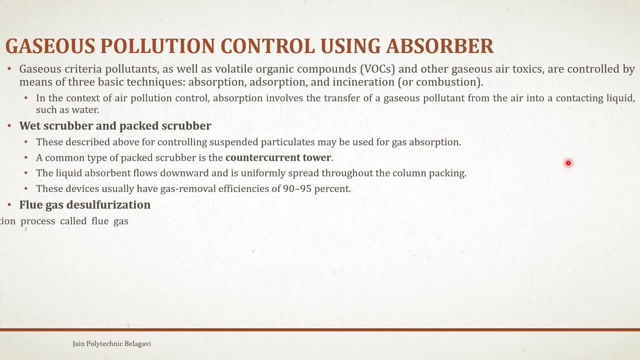 We will go to flue gas desulphurization. The name itself says that the gas, the flue, in the sense it is the bad gas which leads to some of the allergies and the even it leads to the death. We use the sulphur means we use this instrument to desulphurize. 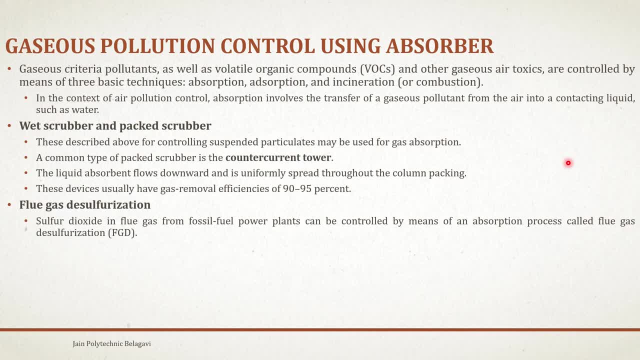 Whatever the sulphur content which has been present in the air, we reduce it using this instrument. The sulphur dioxide in the flue gas from fossil fuel power plants can be controlled by means of an absorption process called flue gas desulphurization. 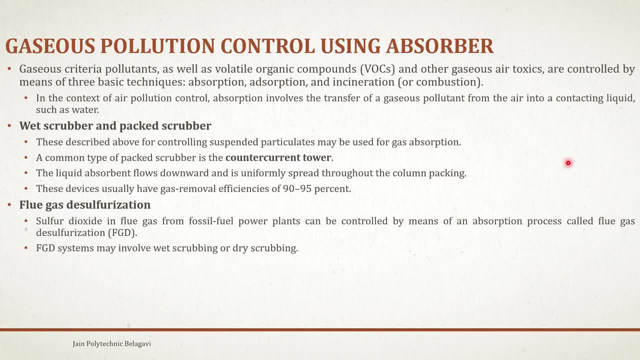 Flue gas desulphurization systems may involve wet scrubbing or dry scrubbing. Among these two, any one, they will be using it for the technique. In wet FGD systems, flue gases are brought in contact with an absorbent, which can be either a liquid or slurry of solid material. 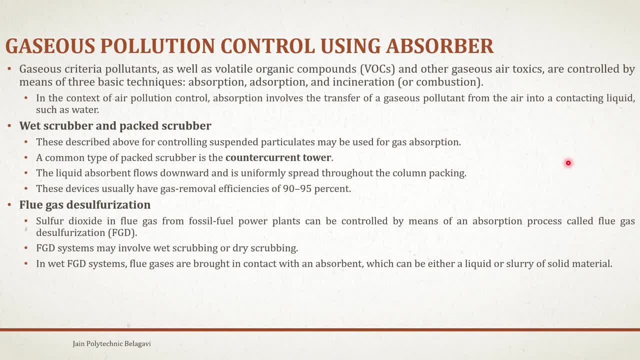 Here the liquid or the medium which absorbs the flue gas. It will be the liquid, purely liquid or slurry, In the sense we are going to add two or more materials to prepare the liquid of the solid material In dry FGD systems. the absorbent is dry pulverized lime or limestone. 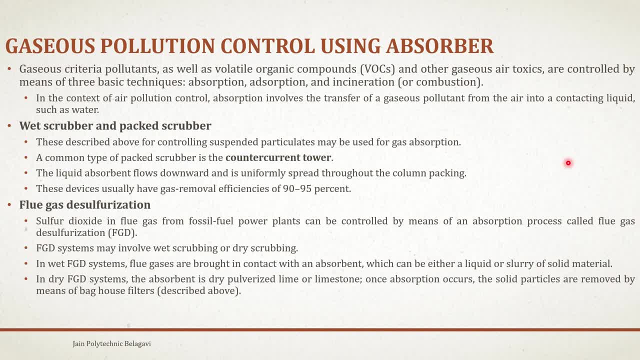 Once absorption occurs, the solid particles are removed by means of bag-house filters In the dry FGD system. the absorbent occurs. The absorbent is lime or limestone and the flue gas. whatever the waste gas, it will be passing through it and it will be absorbed. 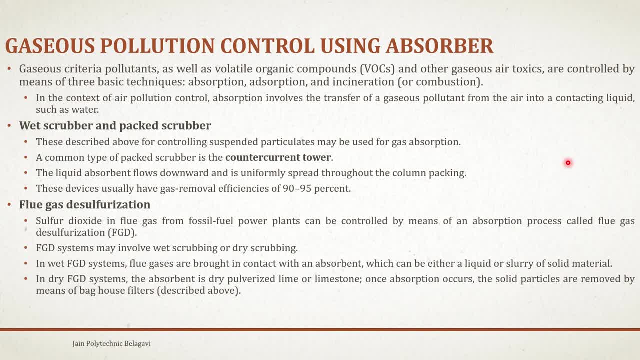 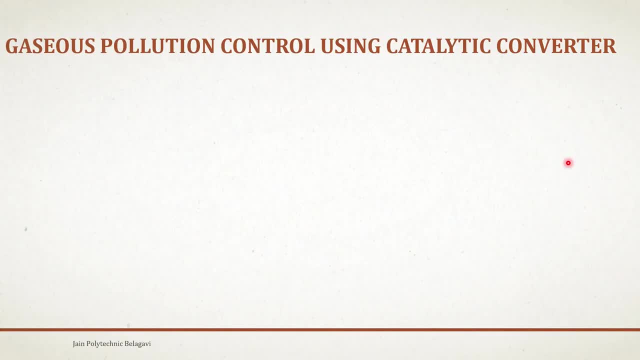 And whatever the material which has been absorbed, that material, we will be separating it by bag-house filtration. Next we will be watching. what are these gaseous? pollution control using catalytic converter. A catalytic converter is an exhaust emission control device that produces toxic gases and pollutants in exhaust gas from an internal combustion engine by catalyzing a redox reaction. 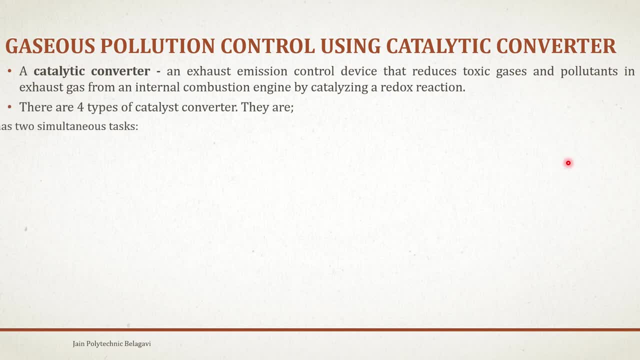 There are four types of catalytic converter. They are two-way- two-way in the sense. oxidation, sometimes called as oxycat. Catalytic converter has two simultaneous tasks. One is oxidation of carbon monoxide to carbon dioxide: 2CO plus O2, will give you 2CO2.. 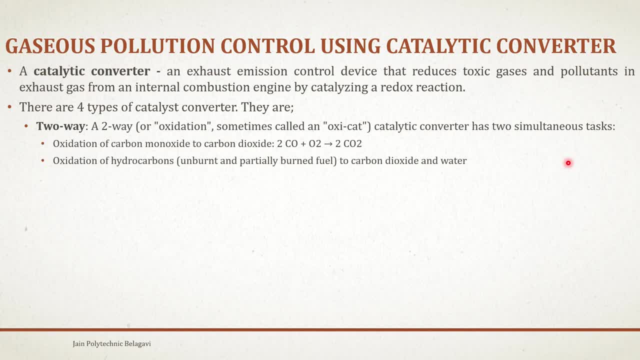 Similarly, the oxidation of hydrocarbons, which is unburnt and partially burnt fuel, to carbon dioxide and water, Just like CXH2X plus CO2.. 2X plus 2 plus 3X plus 1 by 2 times O2 will give you X times CO2 plus X plus 1 times H2O. 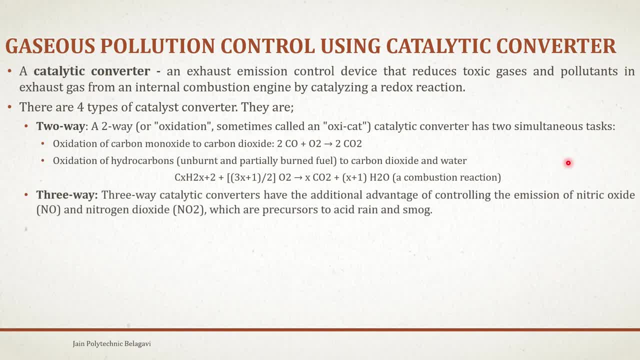 It is the combustion reaction. Next, there is three-way. This three-way catalytic converter has the additional advantage of controlling the emission of nitric oxide and nitrogen dioxide, Which are precursors to acid rain and snow. These are the two gaseous pollutants which leads to acidic rain, as well as with the company of sulfuric acid. 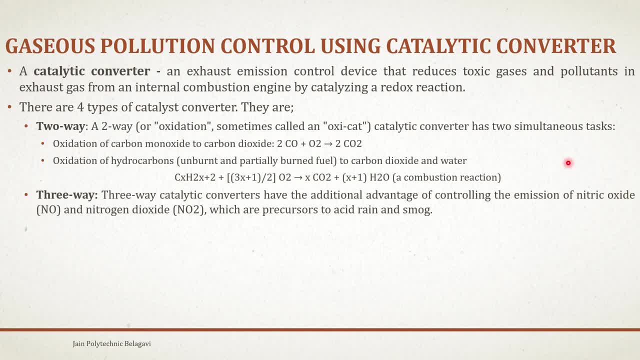 And this three-way catalytic converter will help in reducing these two gaseous pollutants from the air. And next, diesel engines. for compression ignition in diesel engines, The most commonly used catalytic converter is the diesel oxidation catalyst. This might be- you might be studying your science- subject where the diesel engines will help in reducing the oxide fuel fossil fuels oxidation chamber. 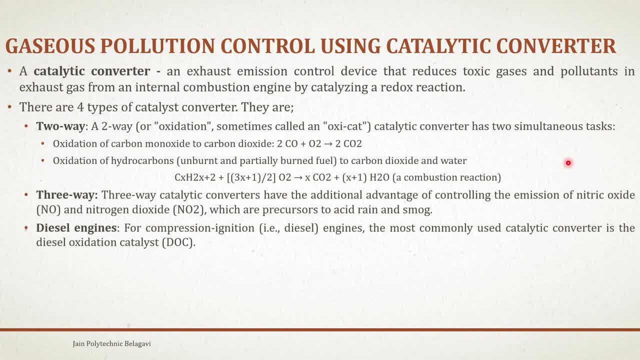 Will help in oxidizing the oxidizing the diesel and will help in converting itself to means when it is being combustible. The byproduct it will be releasing directly as carbon dioxide, not the carbon monoxide. Lean burnt spark ignition engines: These are the different engine instruments which helps in reducing the carbon monoxide as the byproduct.